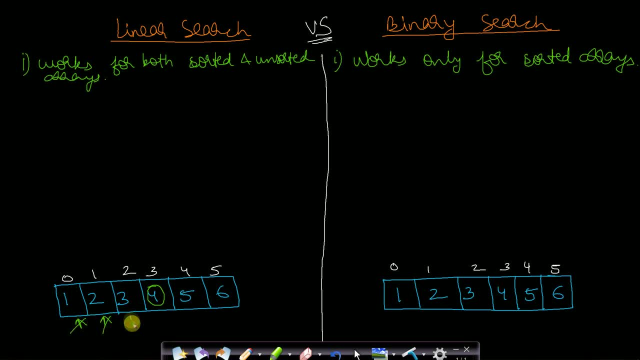 be found, then you will move to the second element, then you will move to third element and, finally, when you find the element, you will stop. This is linear search. What is binary search? When you search for, let us say, element four, then you will take the entire size, the index, of this last one. 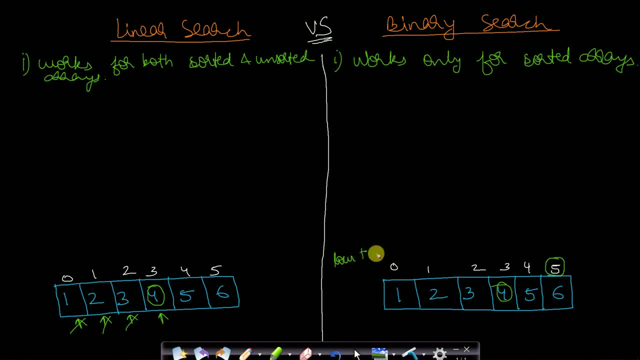 is five. therefore, what you do is you find the middle element, That is equals to low plus high index plus high index by two. Here, low index is zero, high index is five, and zero plus five by two will be equals to two, Removing the fractional part. 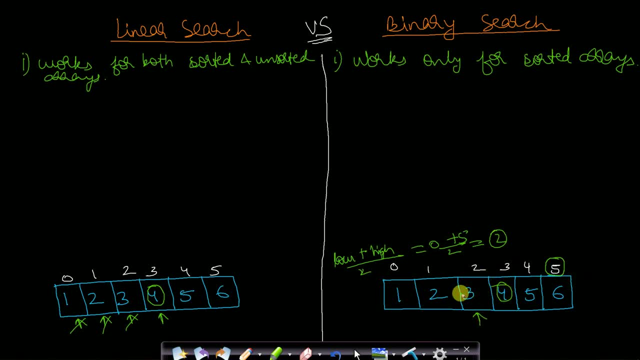 therefore, the middle element will be this one, index two, which is having three. Now, since three is smaller than the element to be found, which is four, and since our elements are arranged in ascending order, therefore, what we will do is we will just discard all these elements and move to the right hand side. Now, the middle element of this right array will be: 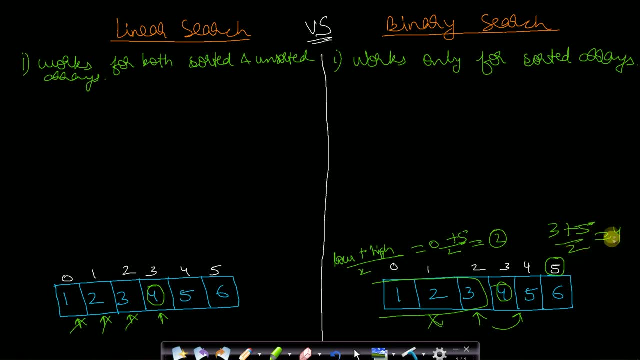 three plus five by two, which will be equals to four. therefore, we will move now to index four. At index four, we will check whether this element five is equals to the element to be found. and we see that it is not equals, but it is greater than the element to be found. So therefore we will move. 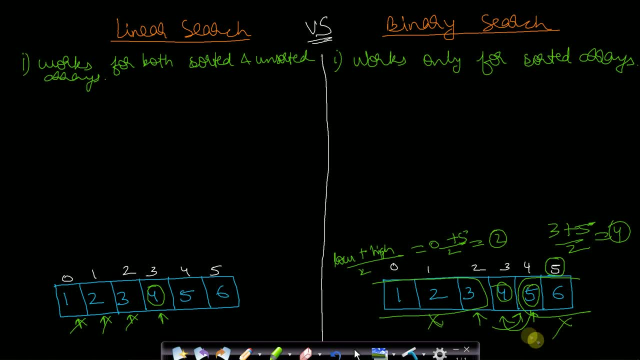 to the left, discarding this entire array. Okay, So now we move to index three, and since we have just a single element in this array, this four will be compared with the element to be found and therefore our element will be found. This is how the binary search works. Therefore, it works only for the sorted arrays and it is not like it. 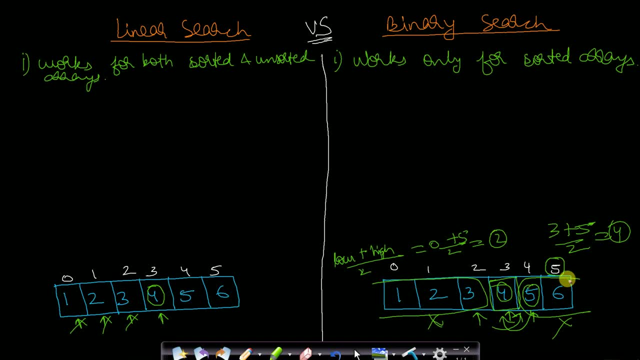 will work only for ascending order elements and will not work for descending order. It will definitely work for descending order. You will just have to tweak a little in your code. Okay, Therefore, you can see that the time complexity of the linear search here in our binary search is the order it will be. 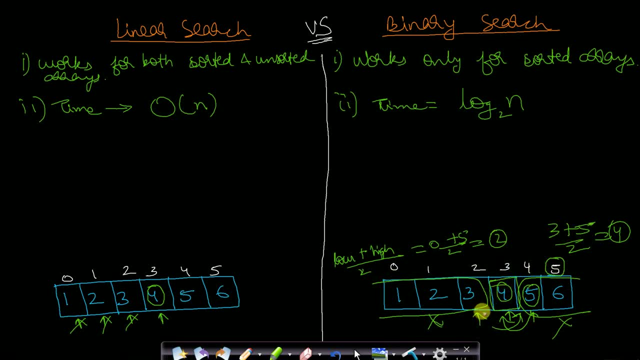 good number 0, then the correct order would be G. Now the number of searches for the line set here has to come from the line set in the left right hand side. So the number of searches for the line set here has to be 10 instead of 15 in case of neue. So out of winter search would.